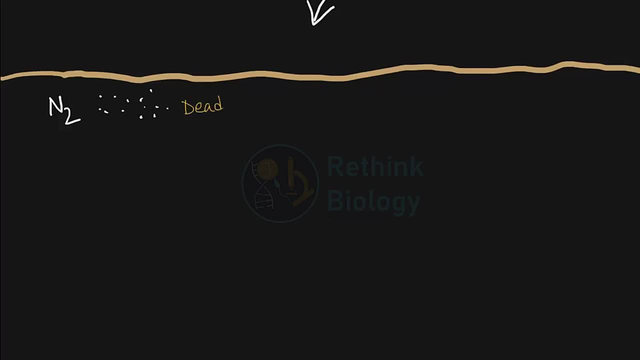 Ammonium ions and nitrate ions are the forms of nitrogen that plants can use. Ammonium ions and nitrate ions are the forms of nitrogen that plants can use. Nitrogen tox delivered from the earlyża of a plant is known as Ammonification. 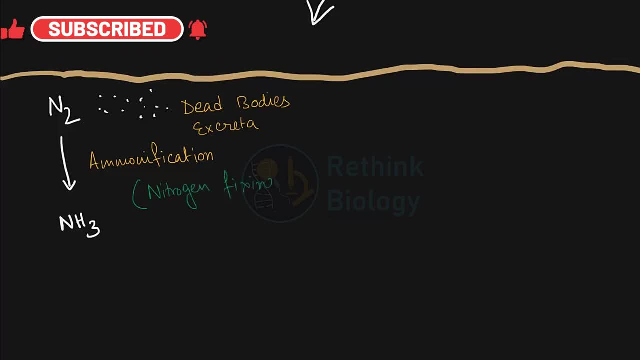 The conversion is mediated by nitrogen fixing bacteria present in the soil. Examples of such bacterias are Azotobacter, Bacillus, Clostridium, etc. 사. The ammonia then picks up hydrogen ion or H plus from the soil to become ammonium or 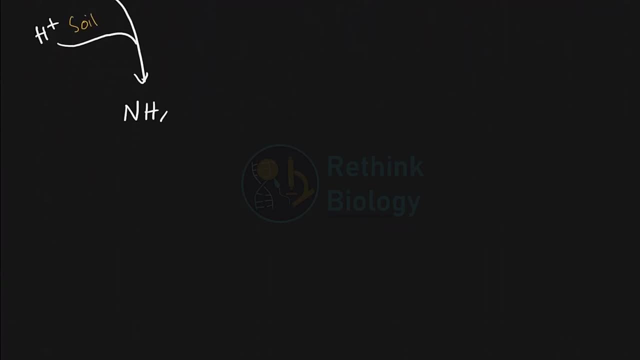 an H4 plus Ammonium can be produced from amino acids of dead plants or animal bodies. The conversion is mediated by ammonifying bacteria, Some examples of which are Bacteria Bacteria, Bacteria Bacteria, Bacteria, Bacillus remorsus. 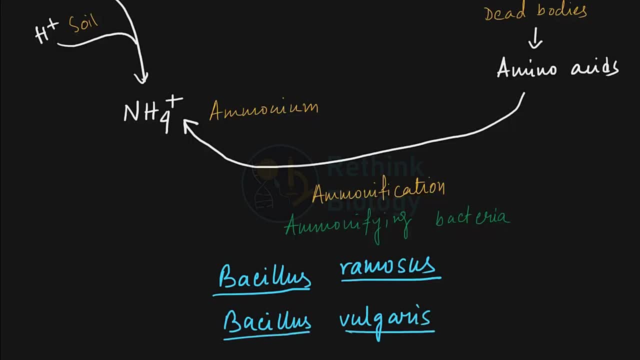 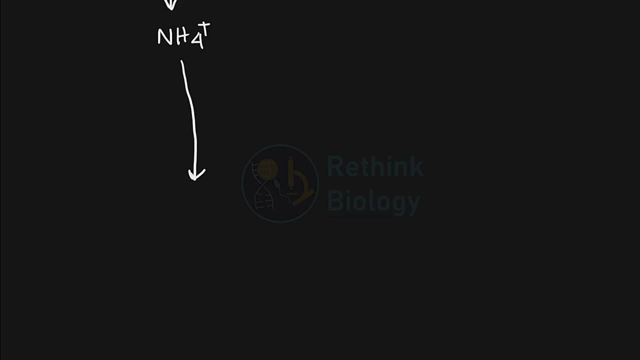 Bacillus vulgaris, The ammonium again converted into nitrate or nitrite by a process known as nitrification. This process is called nitrification. This process is mediated by nitrifying bacteria, Some examples of which are Nitrosomonas Nitrococcas. 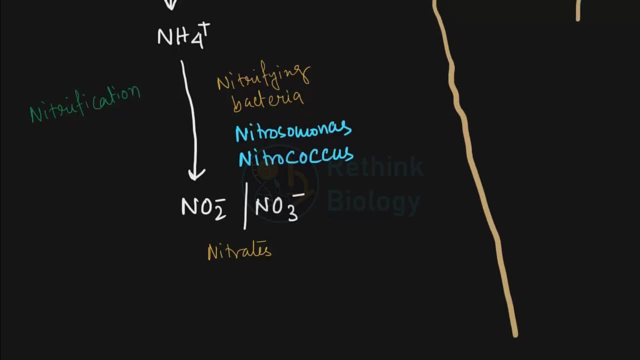 These nitrate and ammonium can be absorbed by the roots of the plants And xylem further transports it to other organs. Some of the nitrates can be further converted into nitrogen. If you happen to have some nitrogen, you can add it.